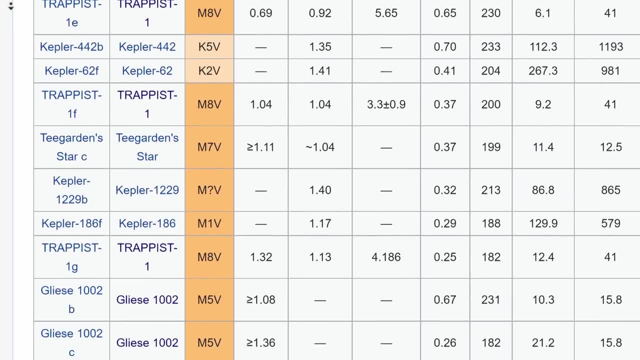 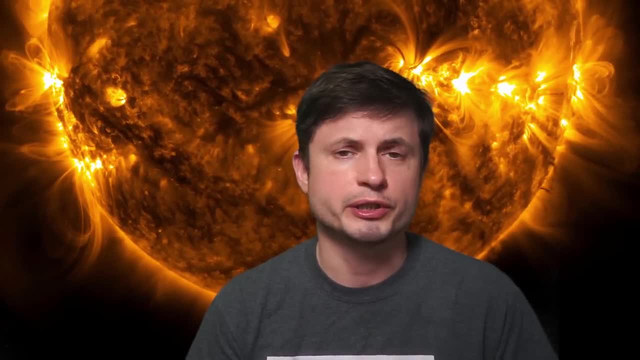 planets seem to be actually orbiting what's known as red dwarf stars, or M-type stars, as they're also known, Stars that we don't really understand very well just yet and that seem to be very different from our own sun, which is a G-type star, But nevertheless, despite all of this, 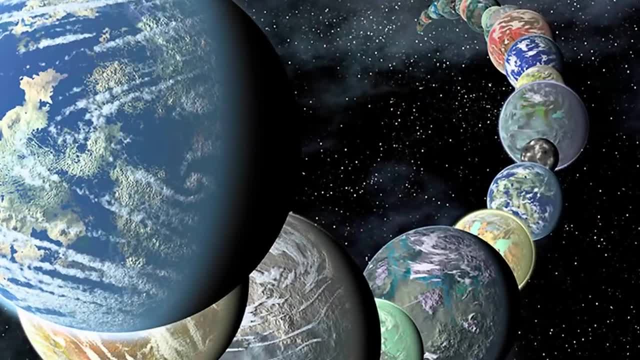 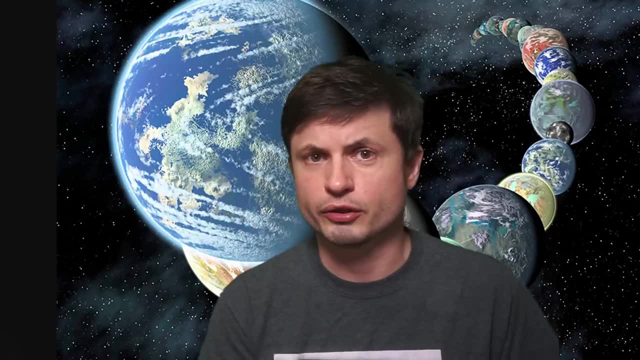 more and more planets are being discovered pretty much every year, suggesting that potentially habitable exoplanets do have a chance to exist somewhere out there. Hello, wonderful person, this is Anton, and today we're going to be discussing the recent announcement of a discovery. 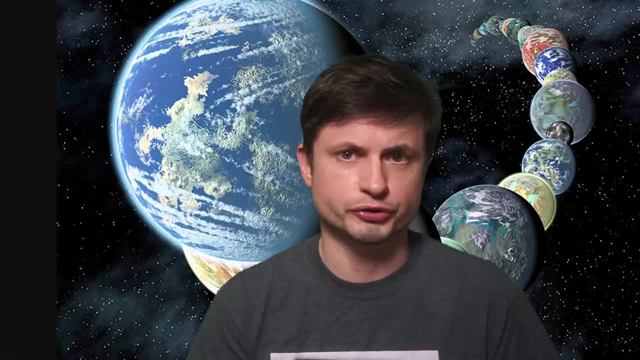 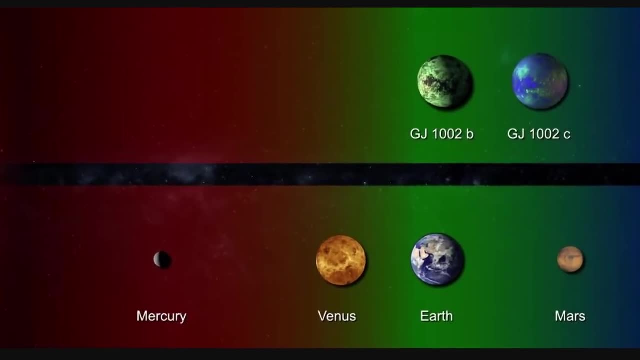 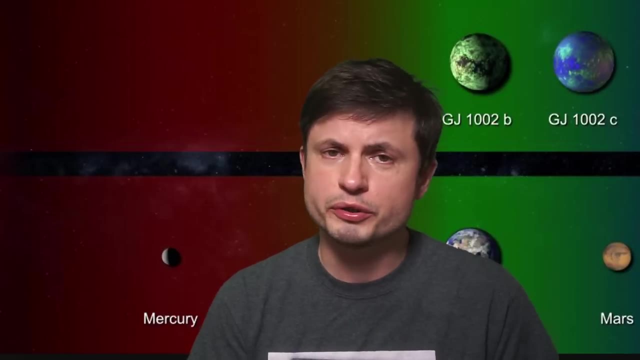 of two more of these unusual planets extremely close to the solar system, making these two planets known as Gliese 1002b and Gliese 1002c some of the most exciting planets in the world. And so today we're going to briefly talk about these two planets, but also discuss another. 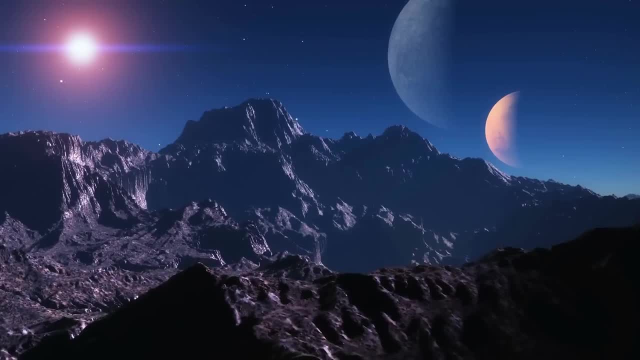 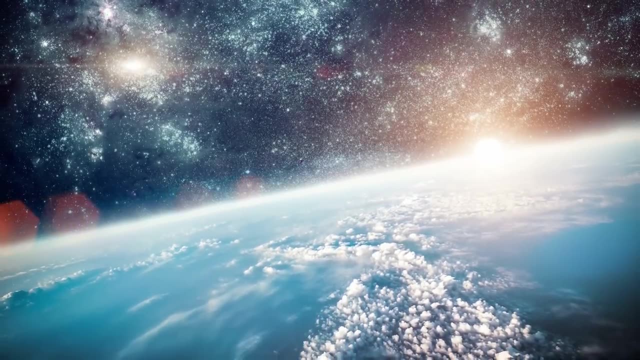 recent paper that essentially tried to create a catalogue that tries to identify which of the exoplanets we've found so far might be the most promising for potential habitability and, of course, for the potential existence of life. But first it's important to understand what the 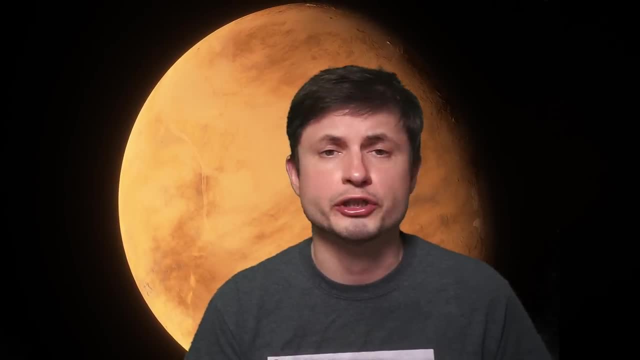 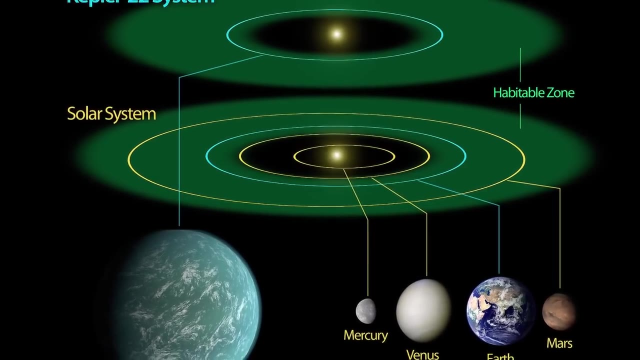 scientists actually mean. when they say habitable exoplanets or potentially habitable exoplanets, It refers to the zone where they were discovered. In other words, based on what we know about the solar system and the location of Venus, Earth and Mars around our Sun, we can generally estimate. 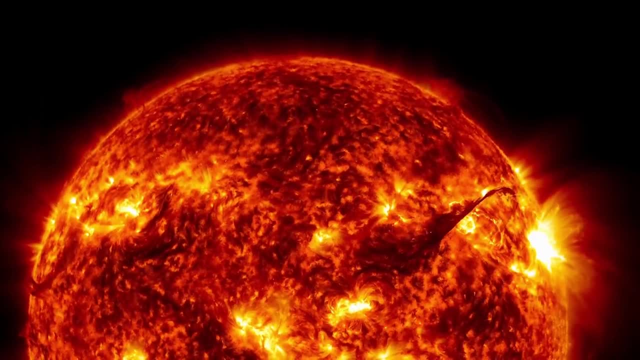 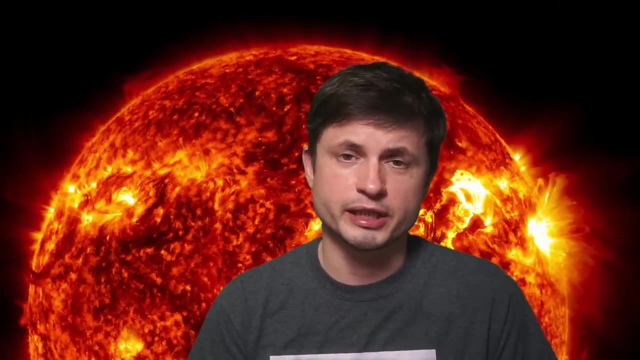 the location in a typical star system where a similar planet might receive similar amount of heat and similar amount of light, And so if any planet with similar atmospheric conditions exists in these zones today, it's assumed that these planets would have an extremely high chance. 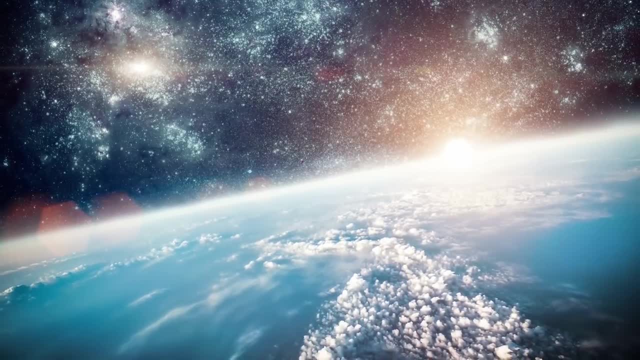 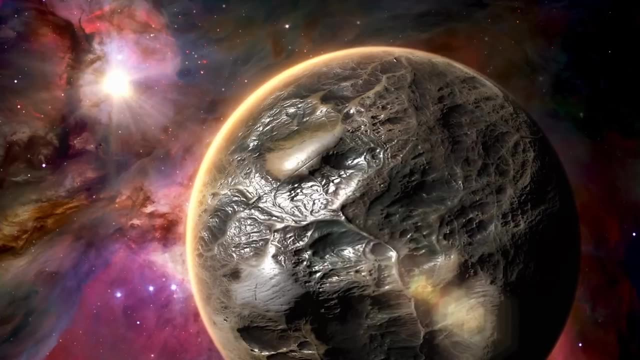 to potentially have liquid oceans and have very similar to Earth's exoplanets, But naturally that's a very big assumption because we don't really know exactly what these planets are like and for all we know, they could be entirely different from anything in the solar. 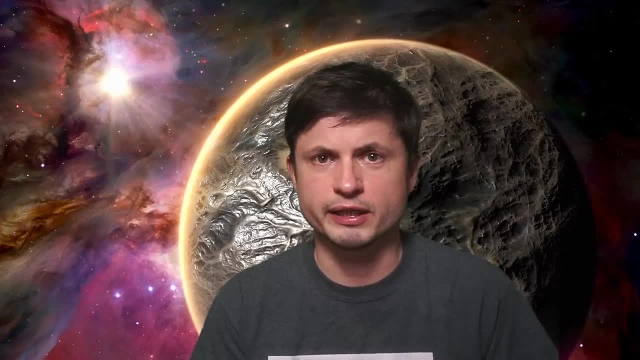 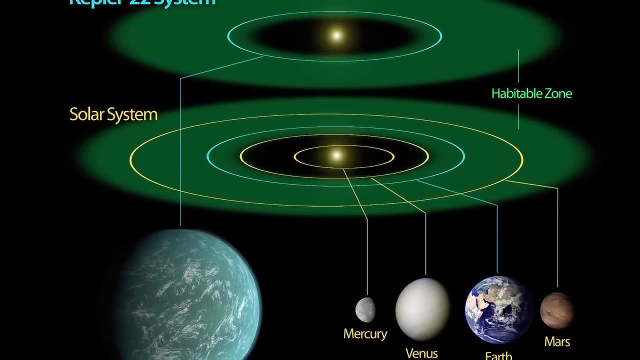 system, But at least for now, it's the only assumption. we can go off until further observations and until future studies. And so since 2014,, since the initial discoveries from the Kepler telescope, in the last 8 years the scientists have been actually finding quite a lot of really. 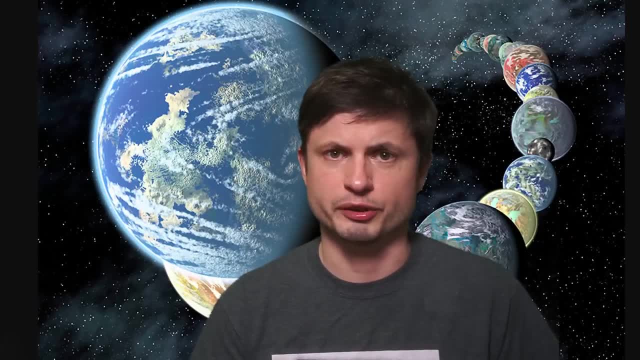 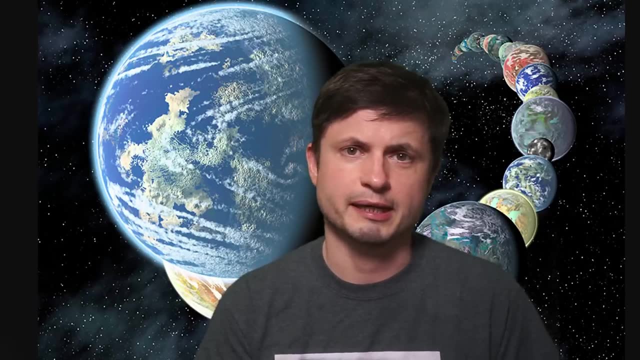 intriguing planets, And the most intriguing one is going to be in a separate video. that's the closest planet to us, Proxima, A planet that's about 4 light years away from us and a planet that's also in the habitable zone. 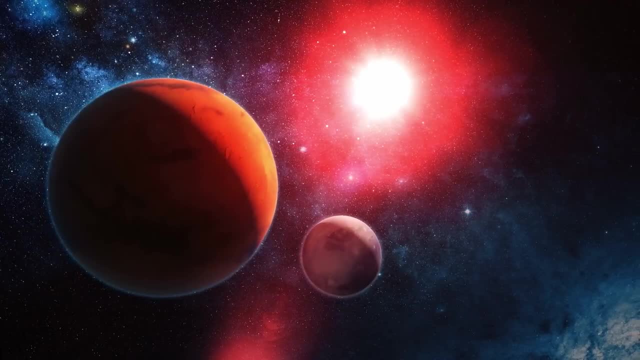 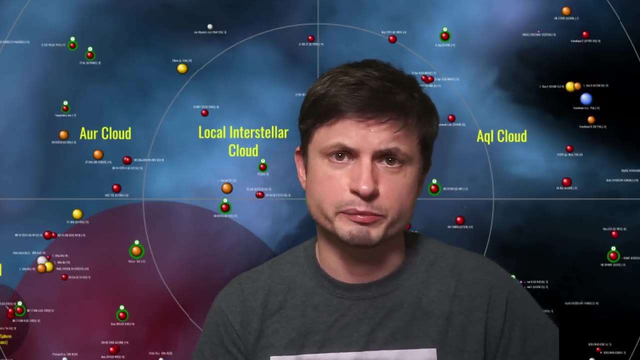 Okay, but what about this new star, The star with two newly discovered planets? Where exactly is it located and what exactly was found there? And just to help you visualize where this particular star is located and where these planets are located as well, here is one of many galactic. 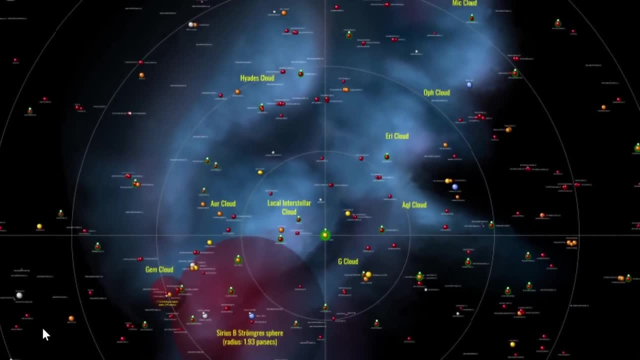 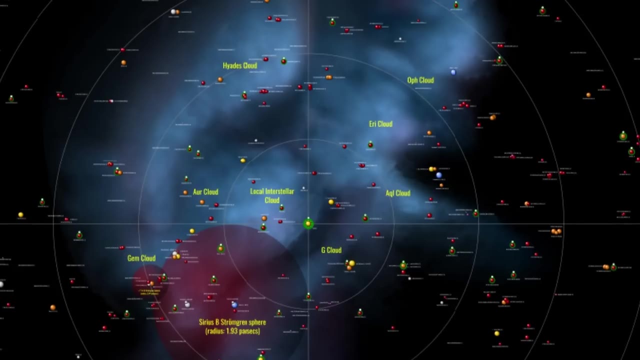 maps I've used previously. that kind of help us understand the number of stars close to the Sun, a distance that's about this far, approximately 16 light years away. As you can see, there are a few dozen stars here, with many of them already known to possess. 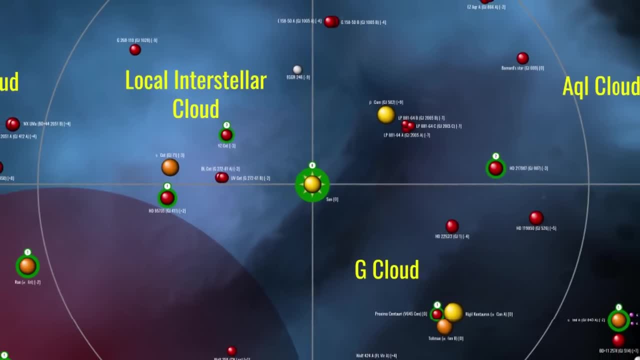 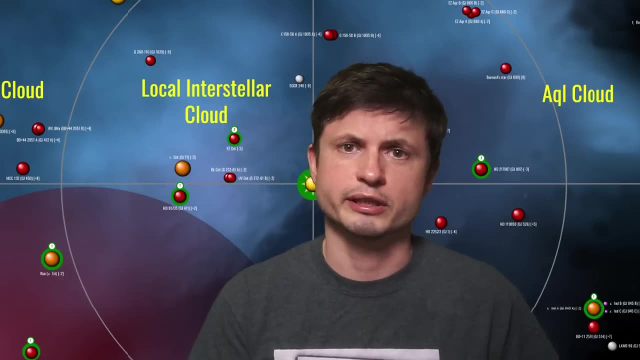 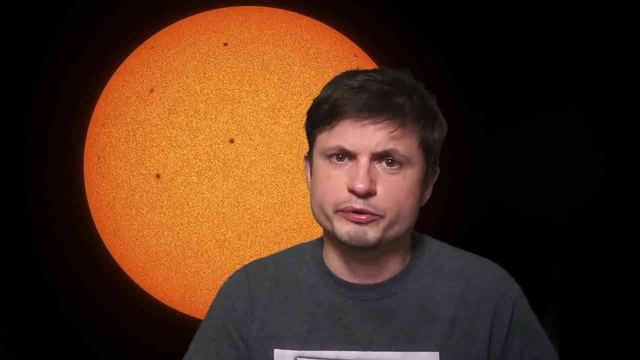 various planets. Naturally, the closest planet, Proxima Centauri, is right here, But at a distance of just 16 light years away from us, there is another, relatively less known star known as Gliese 1002.. A somewhat typical M-type star, or basically a red dwarf, which represent 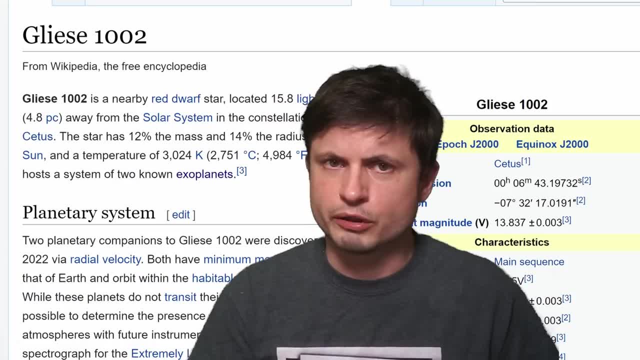 approximately 90% of all stars in our galaxy. Now, originally we didn't really know much about this star, but because it's a red dwarf, we can't say it's a star. But because it's a red dwarf, we can't say it's a star. Now, originally we didn't really know much about this star, but because it's a red dwarf, we can't say it's a star. 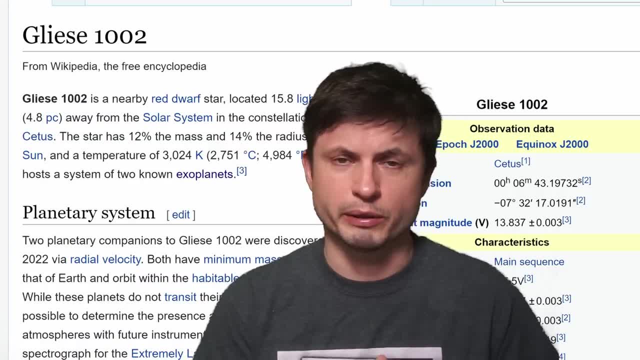 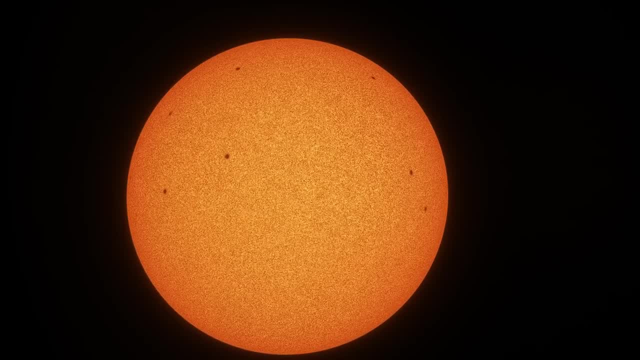 So, in order to see if it's a star, In terms of the actual properties it's about 1 8th the mass of our own Sun and is also much cooler than a lot of other red dwarfs. It also seems to be a lot less active. 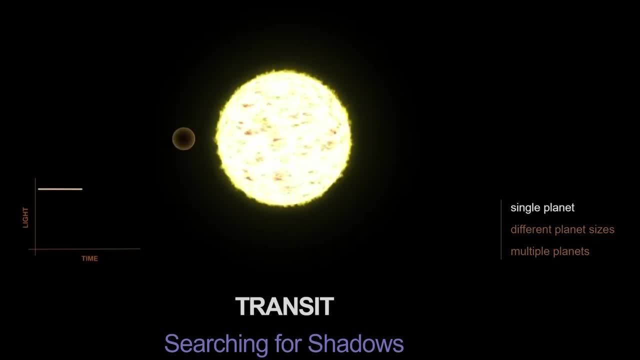 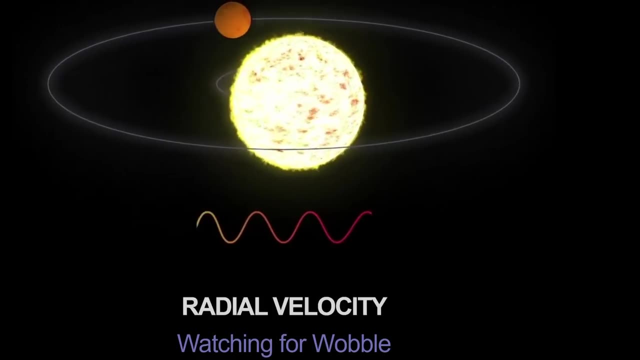 But when looking for various shadows passing in front of the star, so-called transits- the scientists have discovered nothing, And so they actually had to rely on what's known as spectroscopy. they had to look at the star itself and then see how the color of the star 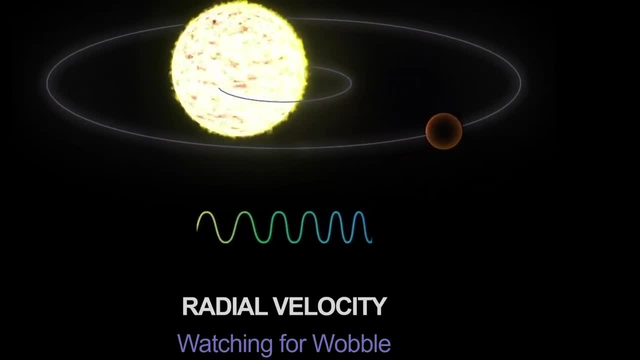 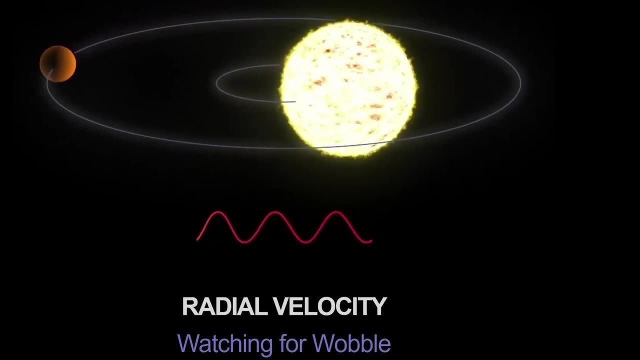 change over time because, as the planet that orbits here pulls at the star, it actually red-shifts and blue-shifts the coloration of the star at regular periods, And for this the scientists used two specific telescopes: the ESO's ESPRESSO and the telescope. 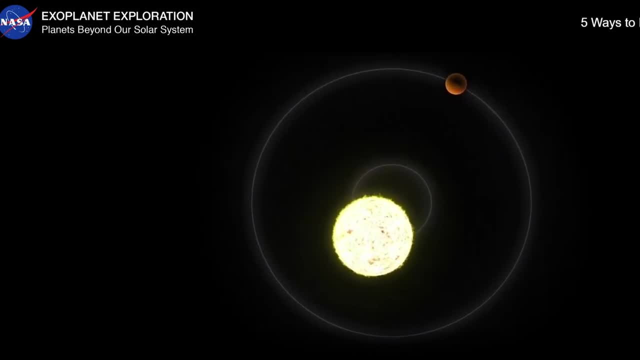 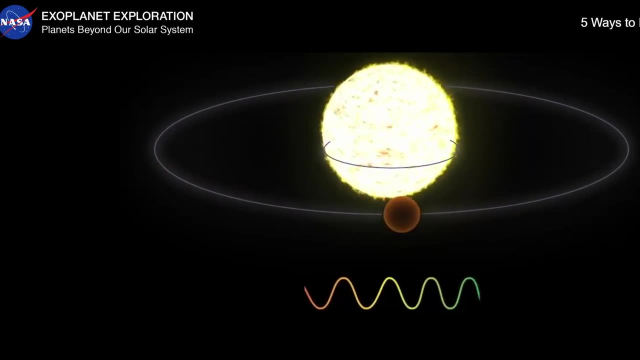 known as CARMENES, And here they looked at the star. for approximately 4 years. they actually had over 130 spectroscopic observations, trying to measure everything as accurately as possible, In the process discovering two separate planets, both in the habitable zone. 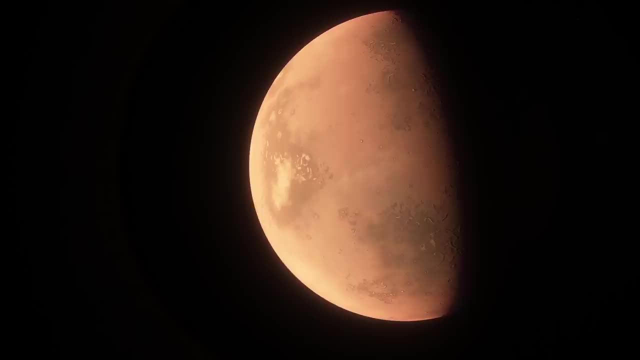 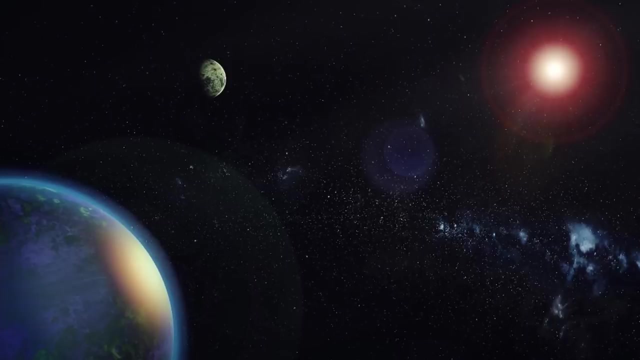 We have the planet Gliese 1000 b and 1000 c. The closest one takes approximately 10 days to orbit, the farther one takes approximately 20 days, With both planets discovered to be relatively similar to Earth, in mass as well, possibly. 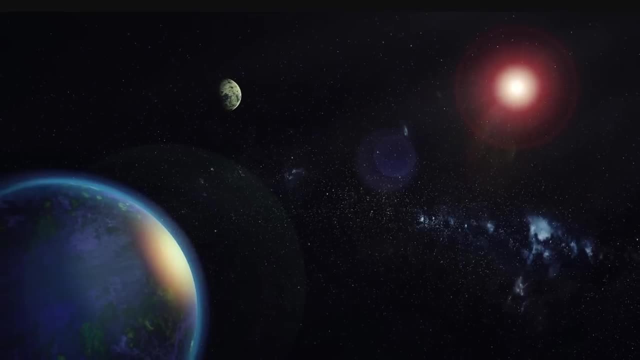 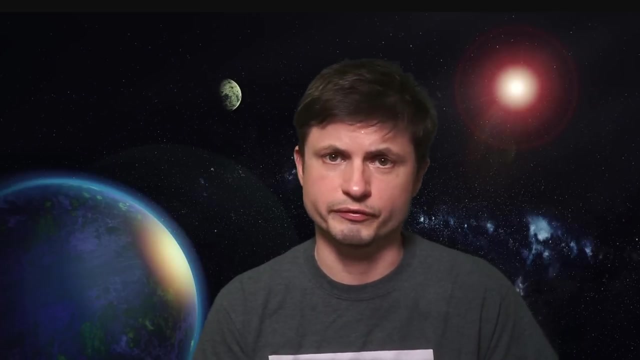 about 8% and 36% more massive. In other words, once again the scientists discovered two extremely Earth-like planets in terms of mass, in the habitable zone of the parent star. And once again, these are extremely close to us- not as close as Proxima Centauri, but 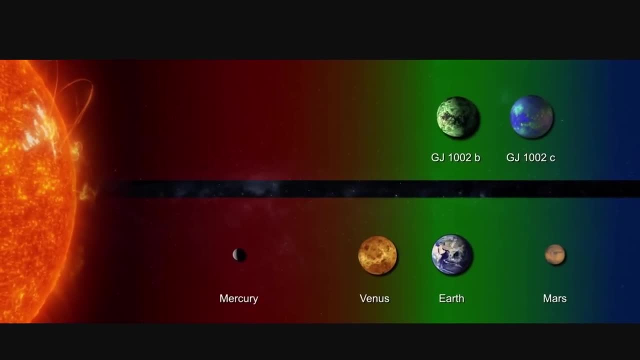 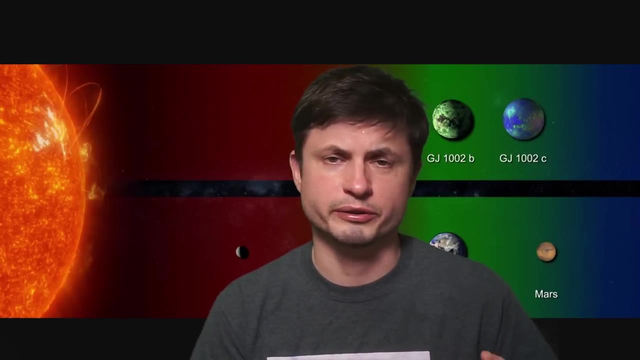 much closer than Trappist-1. But unfortunately, because there are no direct observations of their shadow, it means that we're not going to know their actual size and thus are not going to be able to determine their composition and their density, or even see what their atmospheres are made out of. 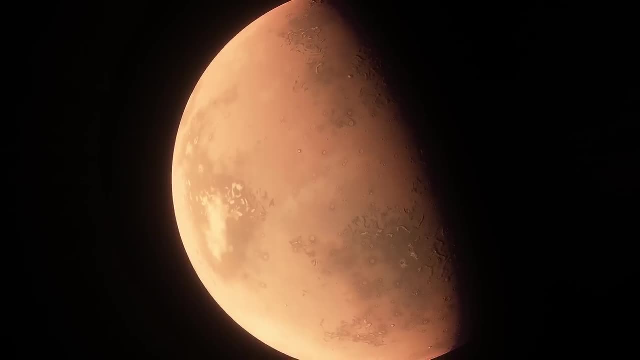 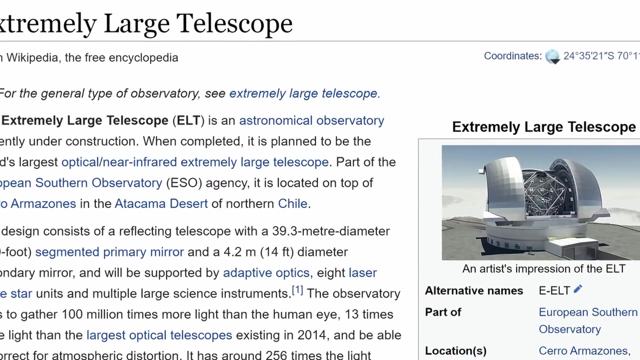 until potential future observations with some of the future telescopes that could maybe see these planets directly and thus assess their atmosphere. At least one of the instruments known as Andes, on top of the extremely large telescope, potentially will have the ability to do this in the next few years. 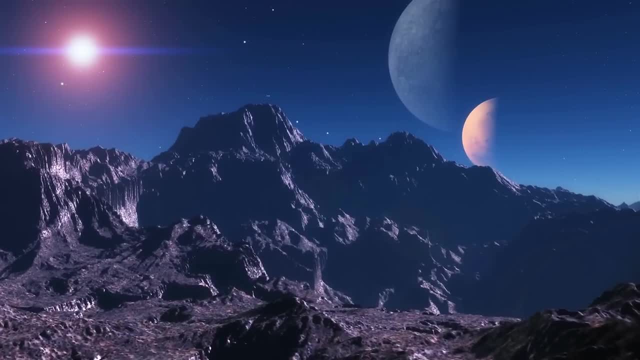 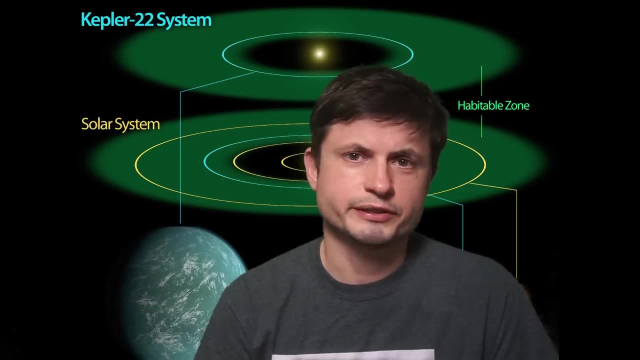 But with the discovery of these two planets we now potentially have seven different planets relatively close to the Sun that seem to be Earth-like enough and seem to be in the habitable zone to, at least in theory, maybe have liquid water and habitable conditions. 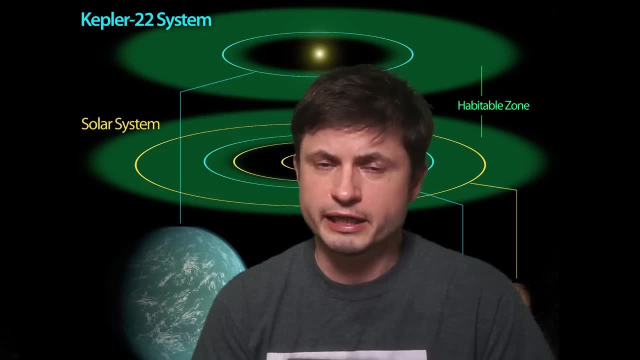 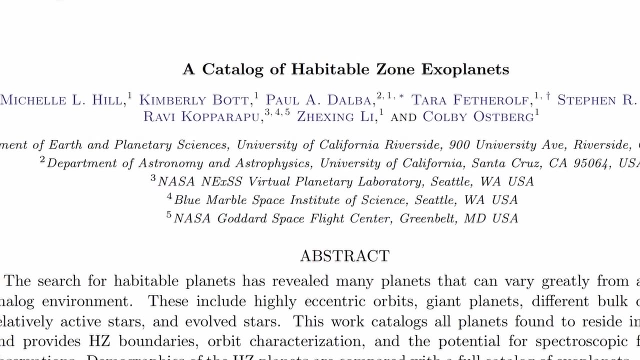 on the surface, And that's why I briefly wanted to mention the other study that actually tries to create the catalog of known exoplanets with potential habitability. The study is also in the description below and in this case it's essentially a catalog. 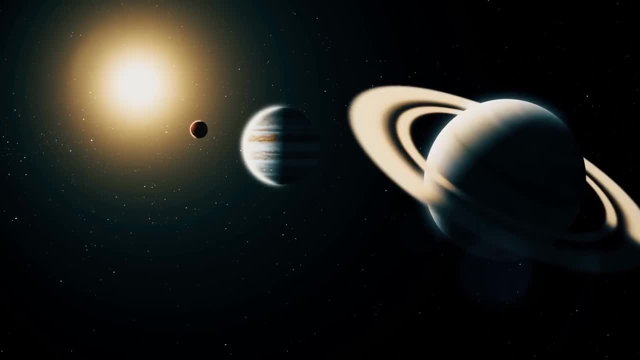 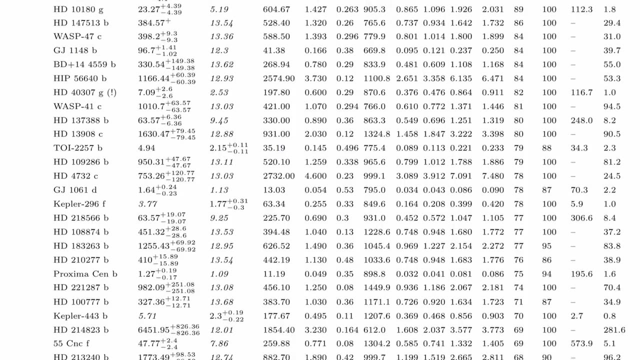 of all of the planets discovered so far. that tries to essentially compare them and potentially discover the planets with the most likely chance for the most habitable conditions on the surface. The study actually goes through a lot of different planets and goes through quite a lot of different. 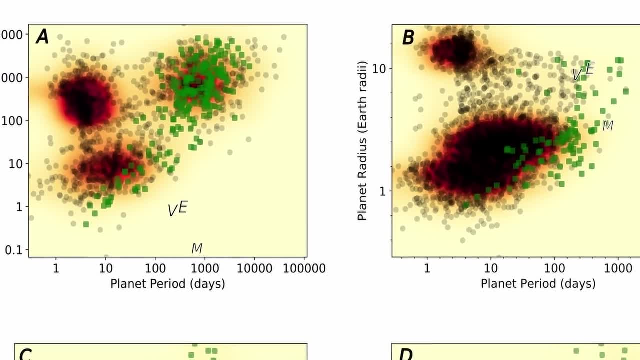 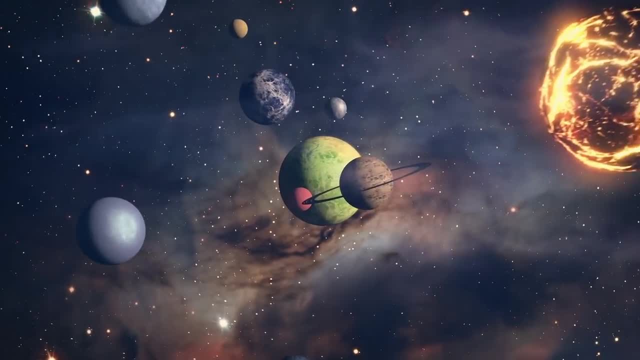 analysis, but in the end only identifies a few of them as the potential habitable candidates, with a few more identified for being just a little bit unusual. So let's get started. And so, just to give you the summary from the study, here are some of the planets, the scientists, 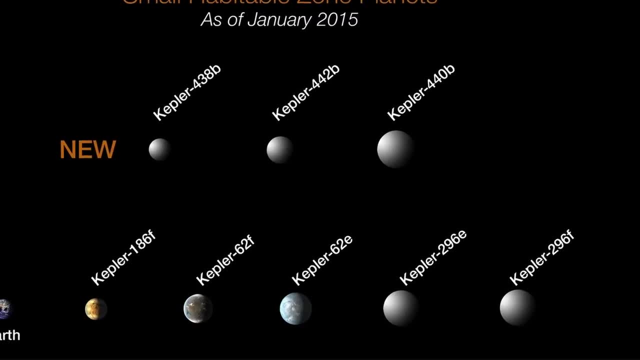 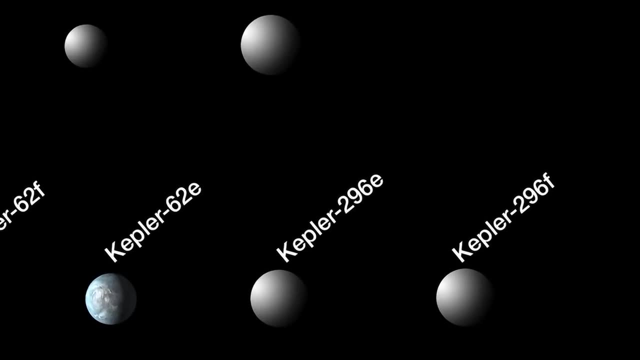 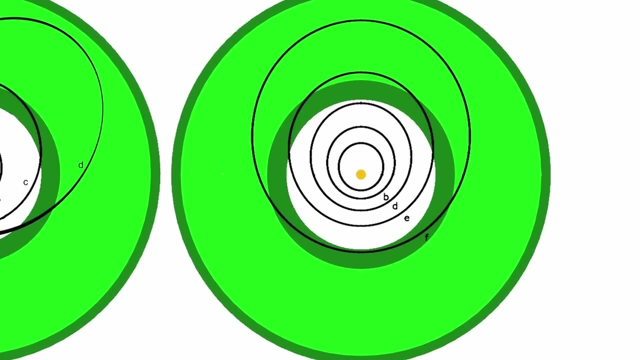 identified as the potential planets of interest. We have Kepler-296f, a planet that spans 100% of its orbit in the habitable zone but seems to have the most eccentric orbit of all of the planets discovered, Which essentially means that it changes the orbit in the star system by quite a large. 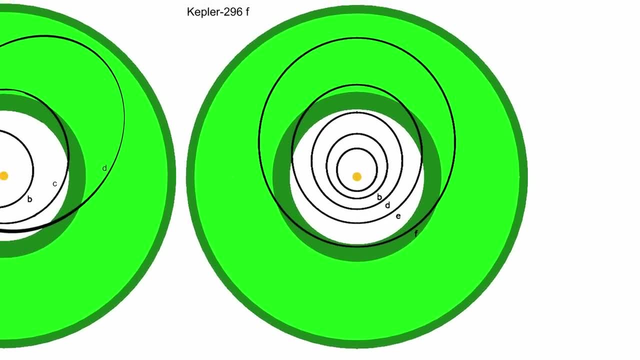 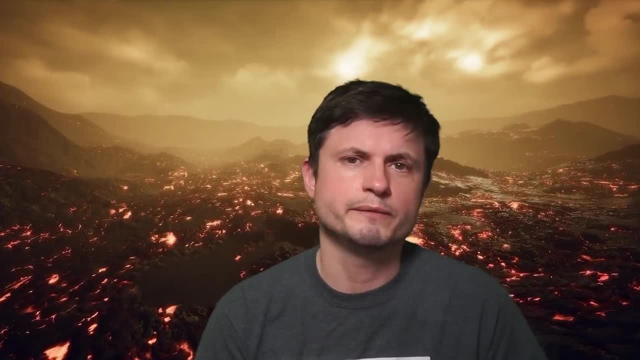 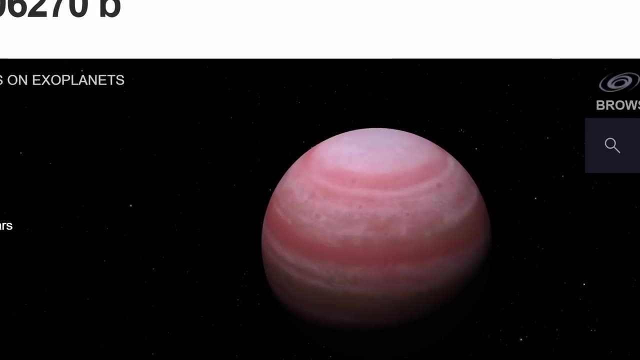 amount and this would probably have very dramatic effects on the planet, including very powerful tidal effects. So this could result in some really high tides, but also extreme volcanism on the surface. We also have planets like HD106270b and HD38529c that seem to be the most massive planets discovered. 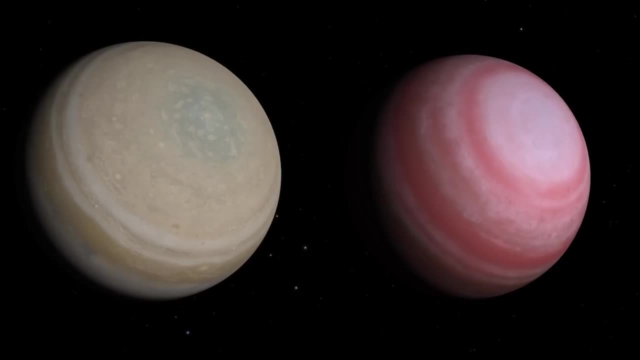 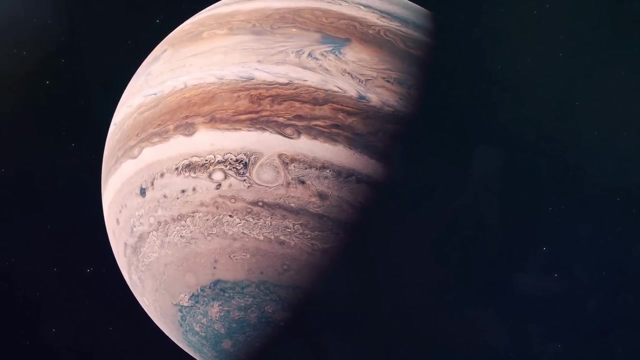 in the habitable zone. These are actually much more massive than Jupiter, in this case being several times the mass of Jupiter itself. But assuming that these planets might have moons, some of the moons around these planets do have a chance to be habitable as well. 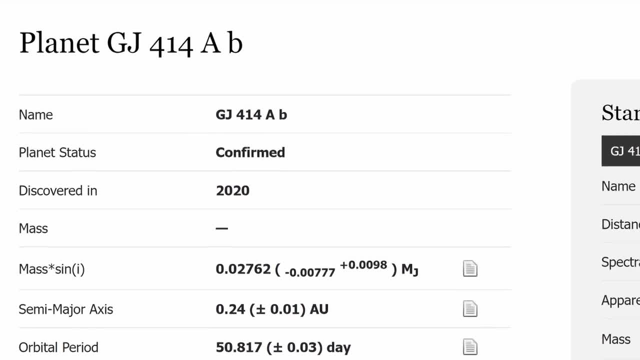 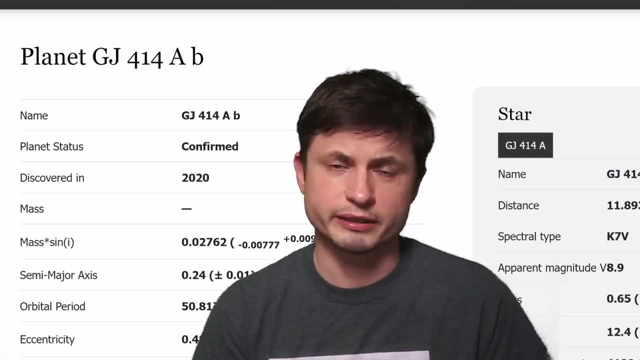 Then there is a really intriguing planet known as Gliese 414ab, a planet around a K-type star, once again in the habitable zone, with a relatively mild star. that's not a red dwarf, with a planet that the scientists want to study more, because it does actually have quite 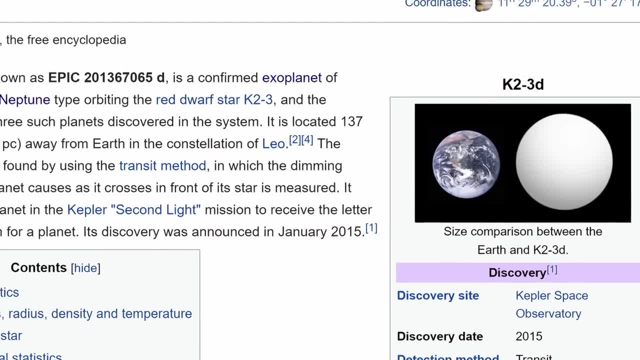 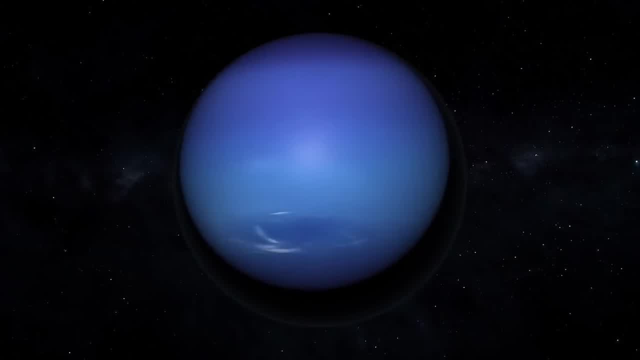 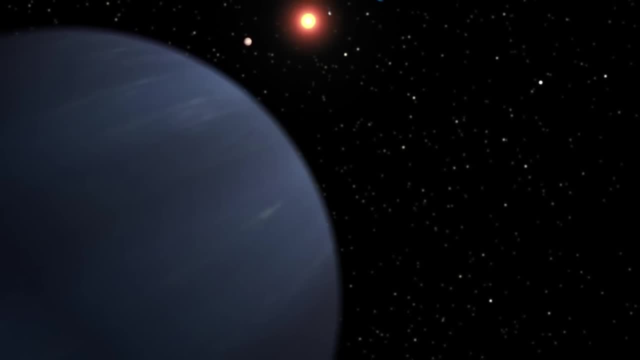 a lot of intriguing properties. We also have planets like Kepler-2 3d, a potential mini-Neptune in the habitable zone, HR4523, that possesses a Neptune-like planet in the habitable zone as well. We also have planets like Mercury-F, a star system that possesses several planets with 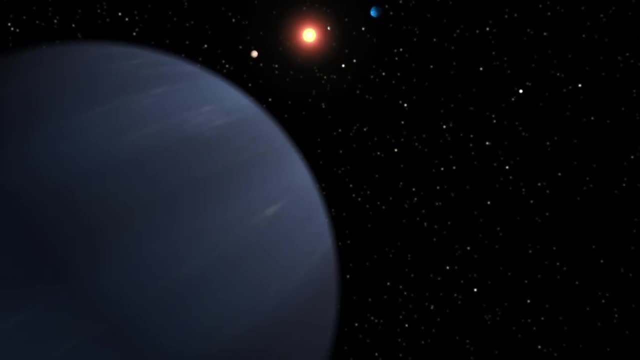 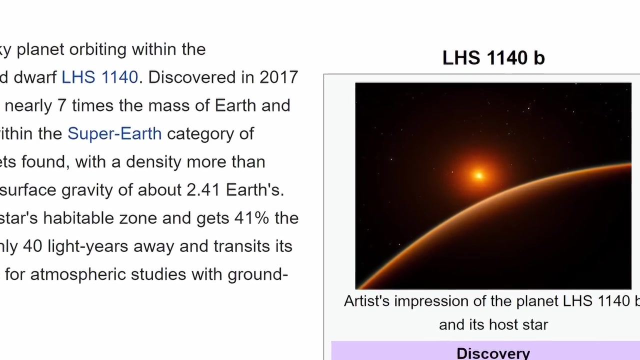 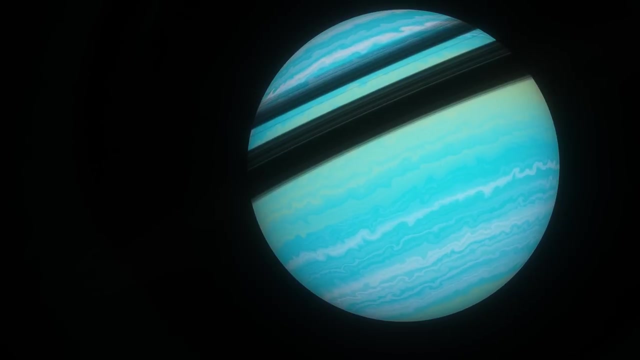 one being extremely hot, but this one being in the habitable zone or potentially some kind of a gas giant. But the most famous planets are LHS1140b, a potentially terrestrial planet in the habitable zone, Trappist-1d, the most Earth-like of the Trappist-1 system, planets Ross 508b. 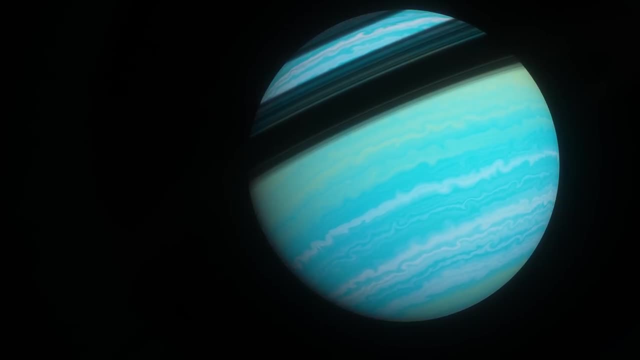 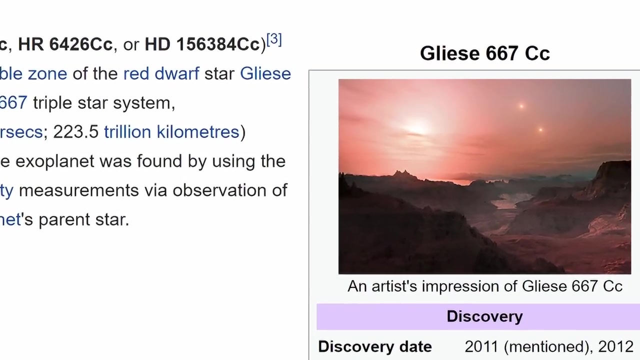 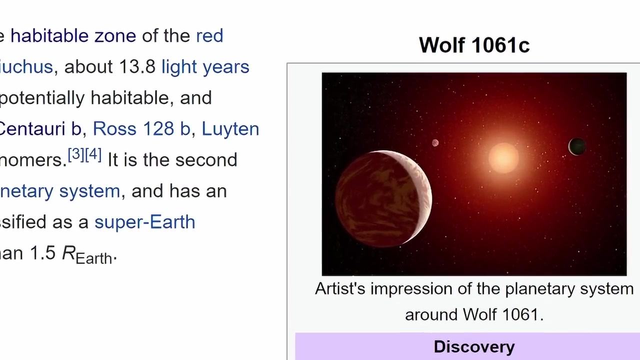 a potentially super-Earth mini-Neptune, or maybe even terrestrial planet in the Ross 508 system, Gliese 614b, Another potentially terrestrial planet around a red dwarf Wolf 1061c. another intriguing exoplanet at a distance of about 14 light-years away from us, Teegarden star b, a planet that's. 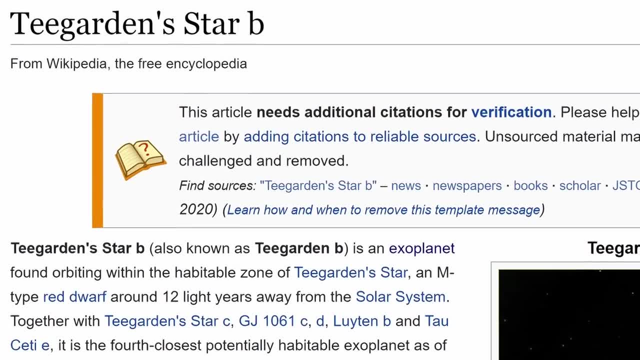 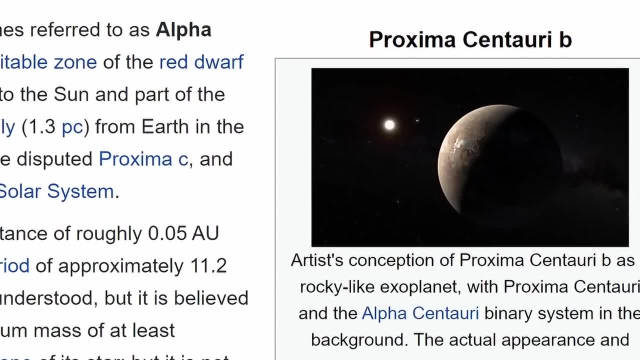 even closer to us once again in the habitable zone, with the distance being 12 light-years. and, lastly, the planet discussed in a separate video, Proxima Centauri b, the closest discovered planet to us around the nearby Proxima Centauri system. 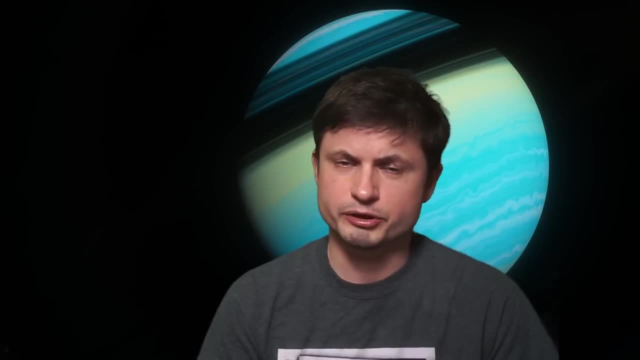 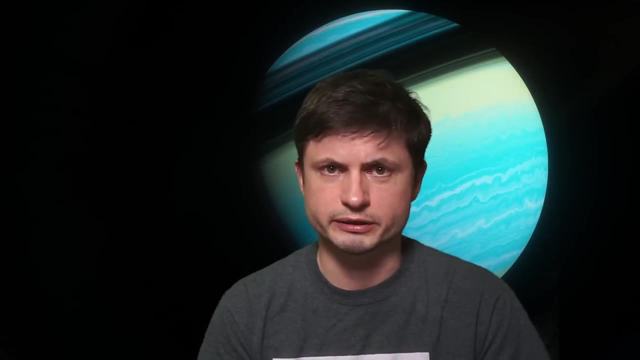 So quite a few of these planets discovered in the last few years. We also have planets that are even closer to us. Some of the planets that have been discovered in the last few years turned out to be very promising for potential habitable conditions, But whether they actually do have these conditions only time will tell. 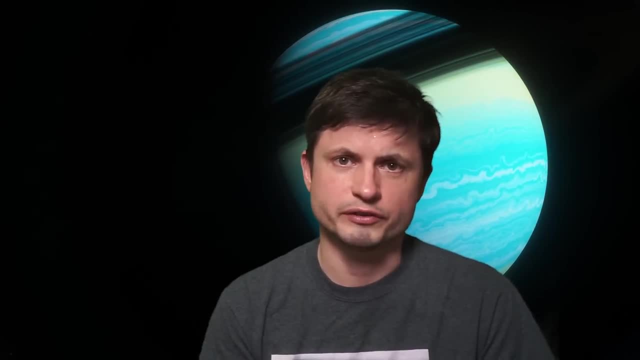 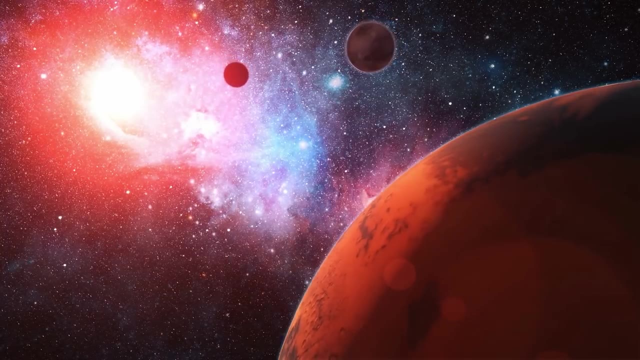 At the moment, a lot of simulations seem to actually suggest that many of these planets might be entirely different from how we imagined them to be, with many of them potentially being completely inhospitable. But until future observations with telescopes like the James Webb that can actually assess. 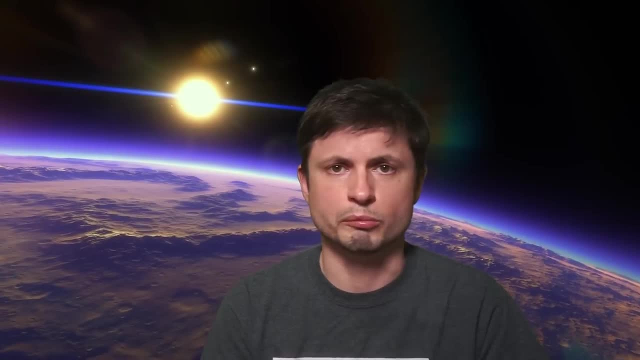 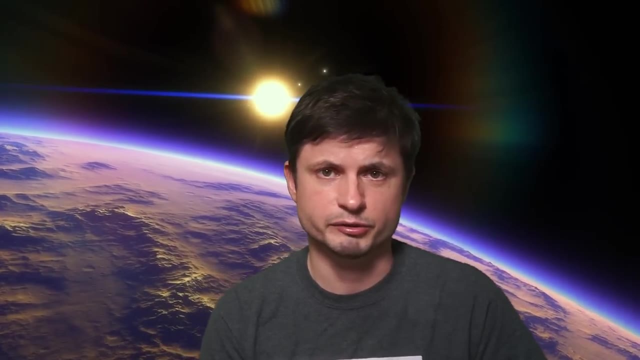 the atmosphere of these planets, we're not going to know much more, Although more details are going to be coming out Sometime in the next few years, And so, until these future discoveries, these are pretty exciting discoveries, but that's pretty much it. 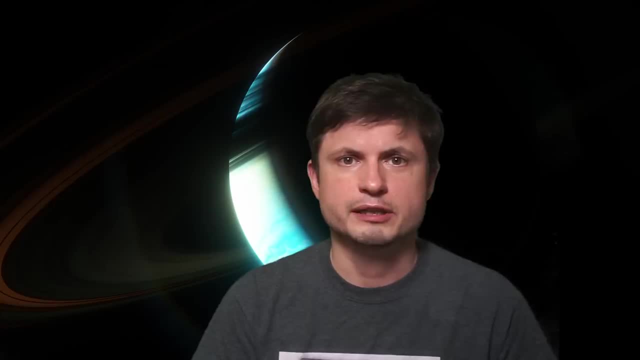 Thank you for watching. subscribe. share this with someone who loves learning about space and sciences. Come back tomorrow to learn something else and maybe support this channel on Patreon by joining a channel membership or by buying the wonderful Burstin t-shirt you can find. 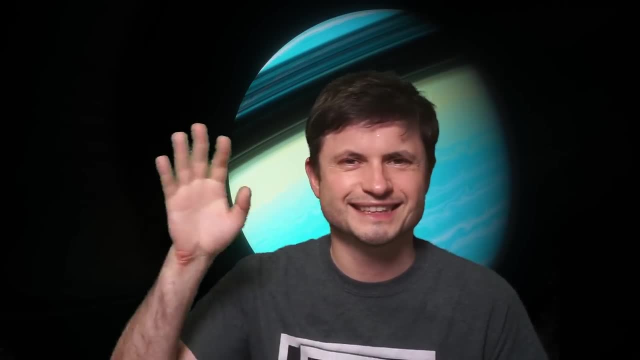 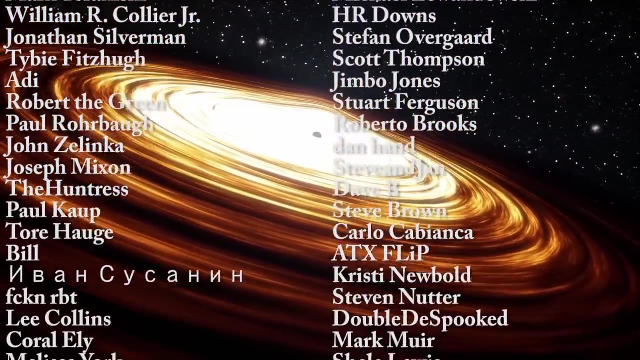 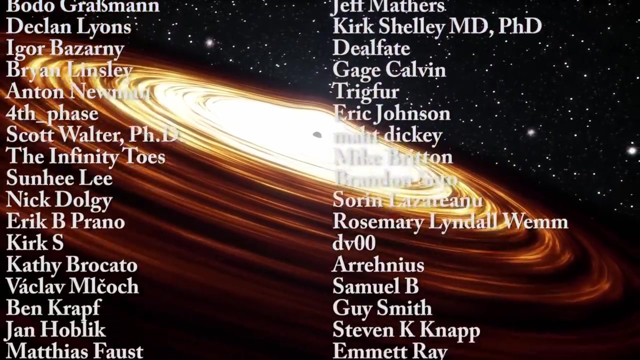 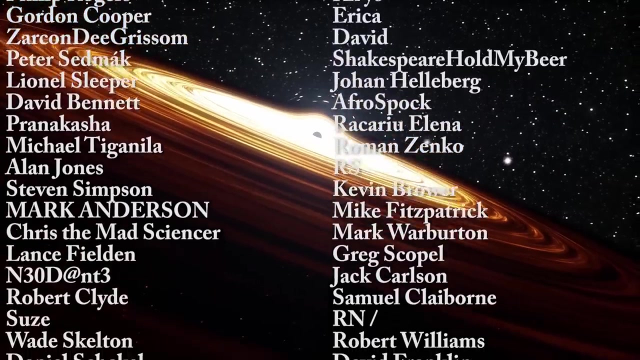 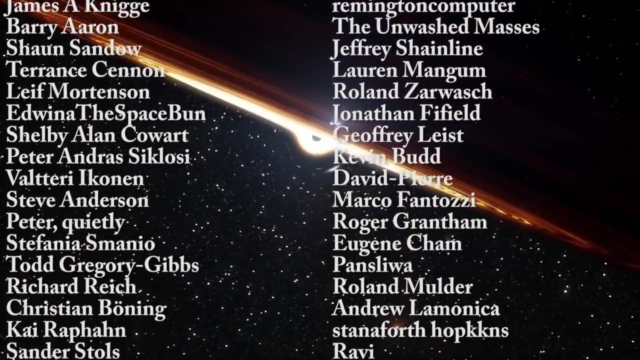 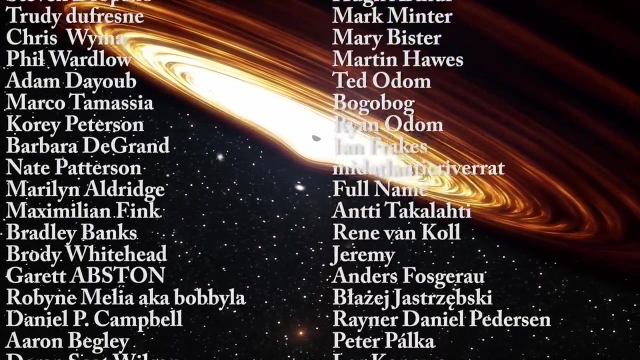 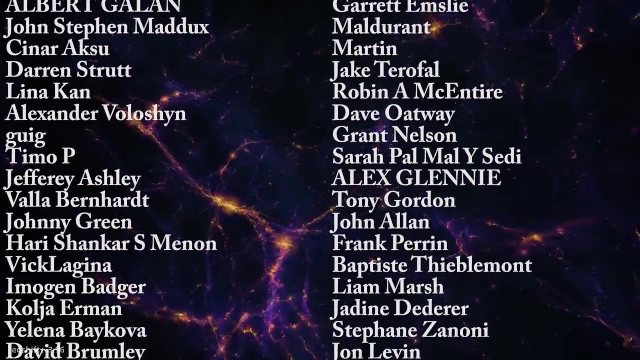 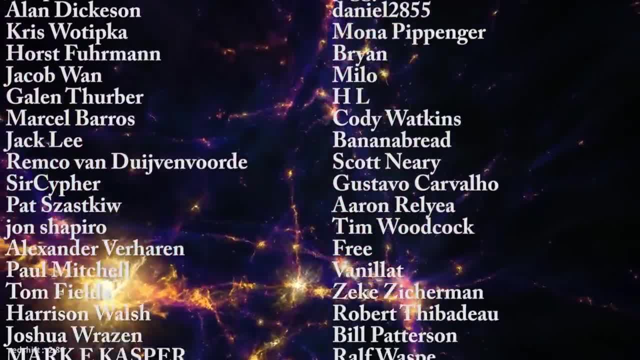 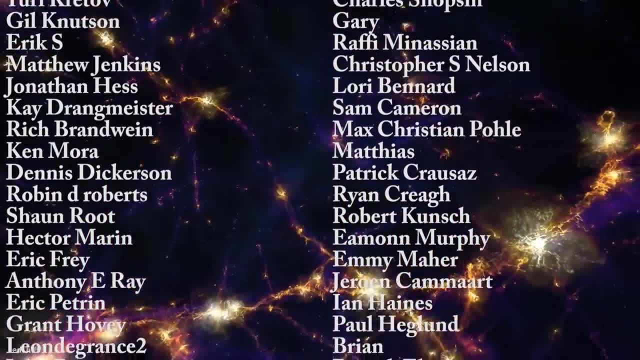 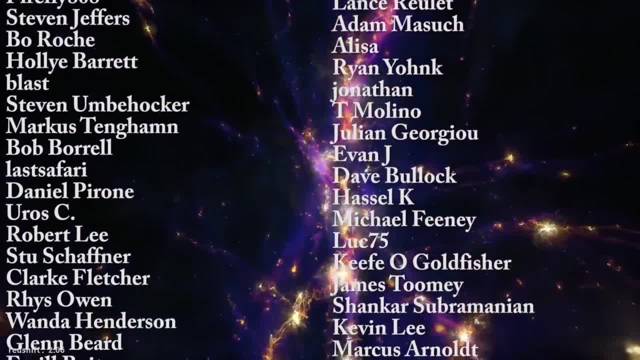 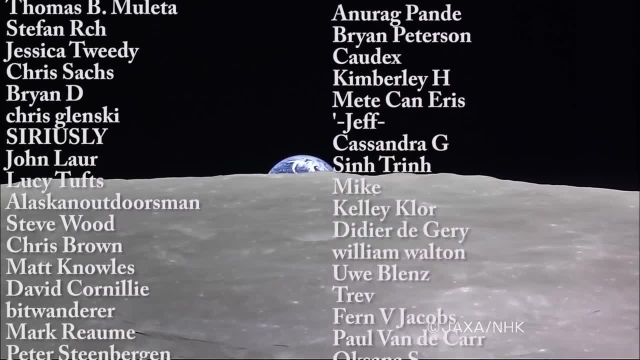